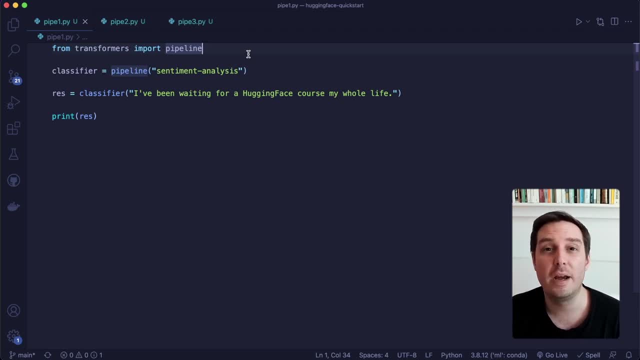 an NLP task because it abstracts a lot of things away for us. And the way it works is that we say from Transformers import pipeline. then we create a pipeline object. So we say classifier equals pipeline, And here we put in a task. 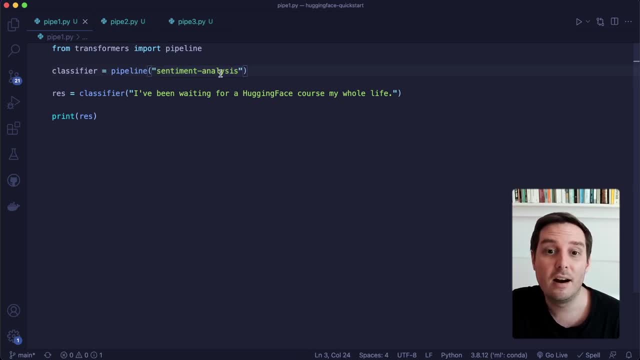 So in this case, to do sentiment analysis. there are a lot of more tasks available and we will have a look at them in a moment, But for now let's do the sentiment analysis. So we create our object and then we. 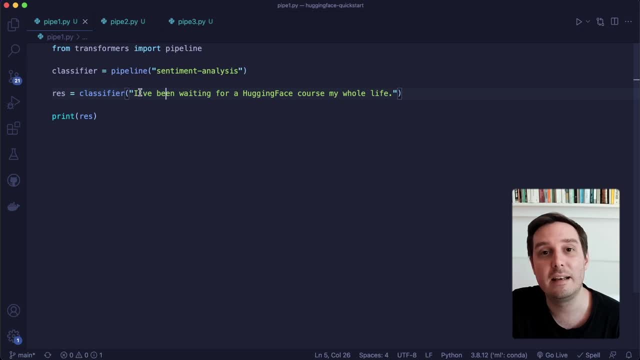 apply this classifier And here we put in the data that we want to test. So in this case, we only put in one string, and the string is: I've been waiting for a hugging face course my whole life, And then we print the results. So now let's run this and see how the result looks like. Alright, and here's. 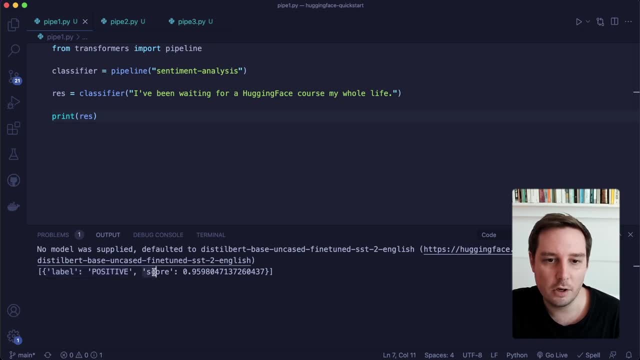 the results. So we see the label which is positive, and we also get a score, So almost 96%. So, yeah, this is super cool And the way this pipeline works is that it will do three things for us. So the first one is the pre processing. So it's pre processing the text. So in this case, 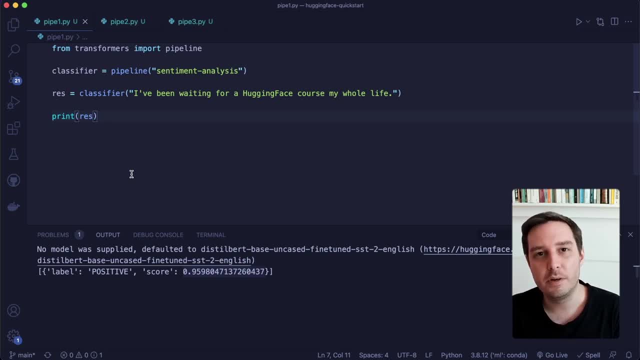 it's applying a tokenizer, then it feeds the pre process text to the model, then it applies the model And then it also does the post processing. So post processing means it will show us the result how we would expect it. So in this case of a sentiment analysis, 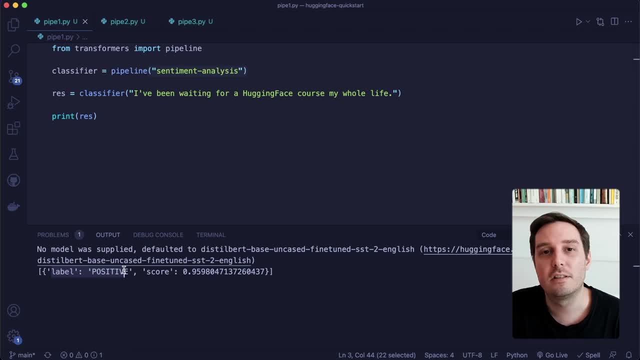 pipeline. it, for example, shows us the label positive or negative, but it can also look different for different tasks. So yeah, that's how it works. And now let's look at a few other examples of pipelines. For example, we can also use a text generation pipeline, And we can also 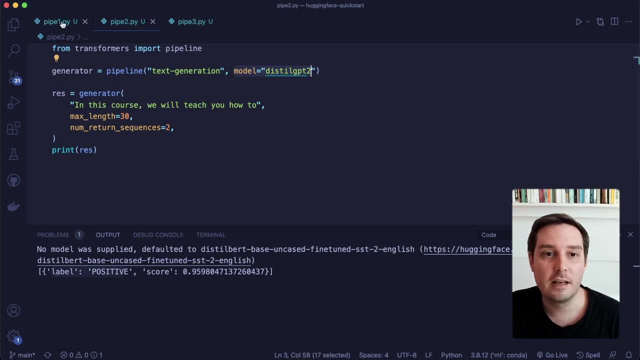 give it a specific model. So in the first example we just use the default model, which you can also see here in the output. But you can give it a specific model, either one that you have saved locally or one from the model hub. So we will also have a look at this in a moment. So, yeah, 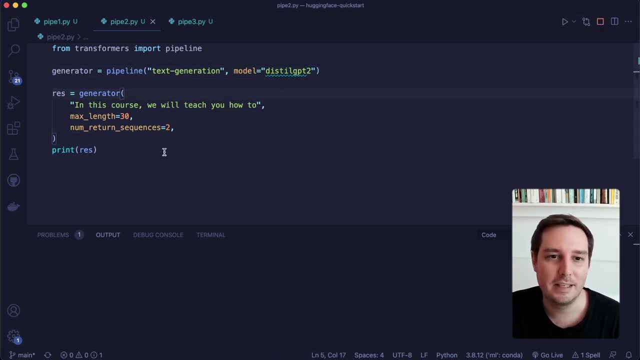 let's apply this example to generate some text, And you can also see there are different available arguments. So for this I just recommend to check out the documentation. So yeah, here's the results. So we wanted to have two possible return sequences. So 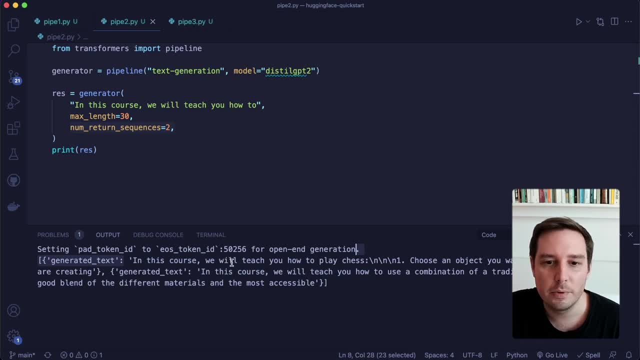 the first generated text is this one: In this course, we will teach you how to play chess. Or here's a second one: In this course, we will teach you how to use a combination of a traditional and simple blah blah blah. So yeah, this also works. And now let's have a look at a third. 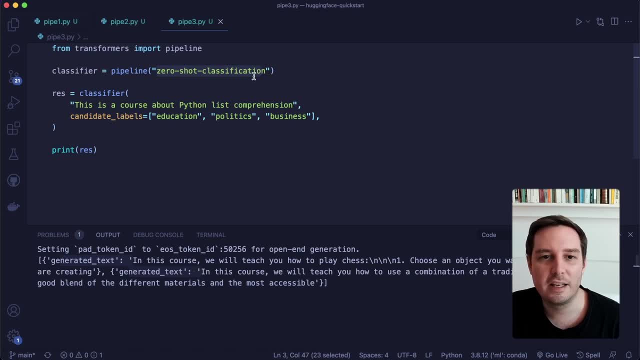 example. For example, we can do zero shot classification. This means we can give it a text without knowing the corresponding label, And then we put different candidate labels. For example, this text can be education, politics or business, And then let's run this and see the result. And here we get the results of all. 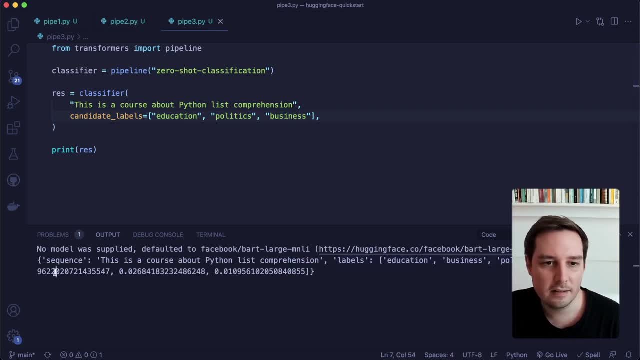 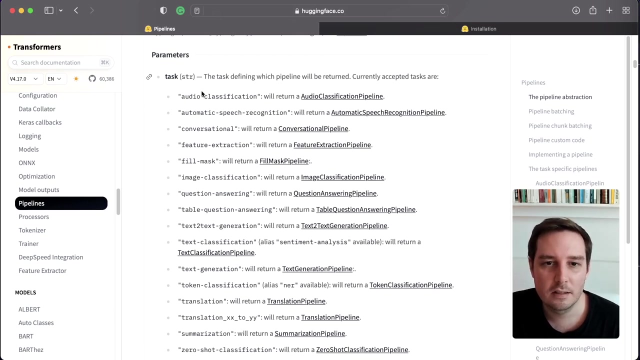 the different labels and the different scores, and the highest scores, with over 96%, is the education which is correct. So let's have a look at the different other available pipelines. So for this I recommend to go to the official documentation, And here you see all the available tasks For 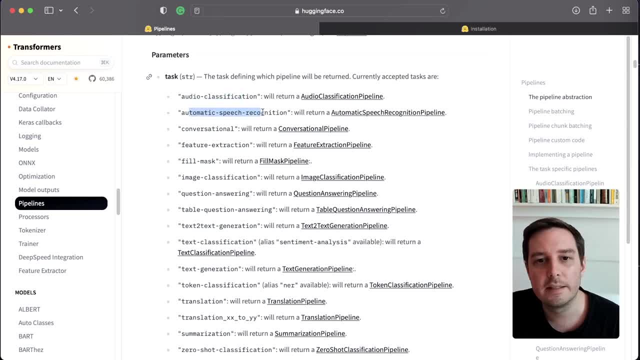 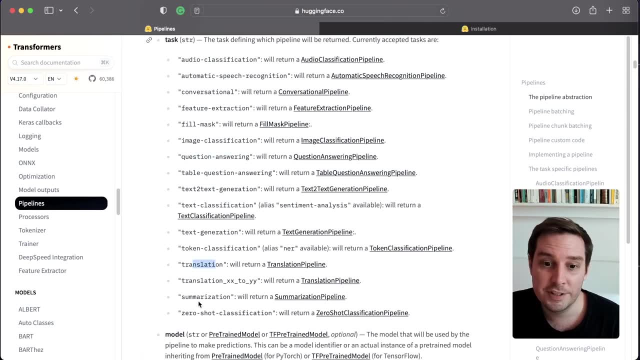 example, we can do audio classification, we can do automatic speech recognition, we can do image classification, question answering and translation summarization. So yeah, this is super cool And yeah, just recommend to play around with different ones and see how it. 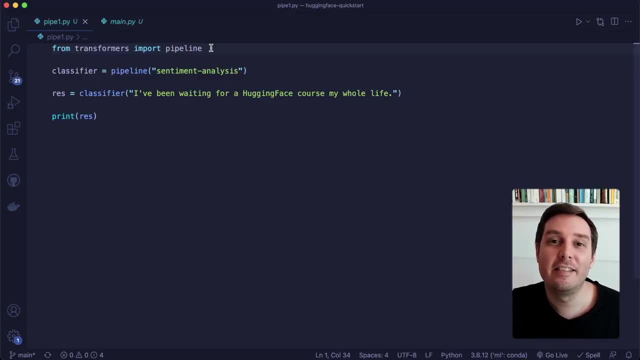 looks like Now let's have a look behind the pipeline and understand the different steps a little bit better. So for this we have a look at a tokenizer and the model class. So we can say: from transformers import auto tokenizer and auto model for sequence classification. 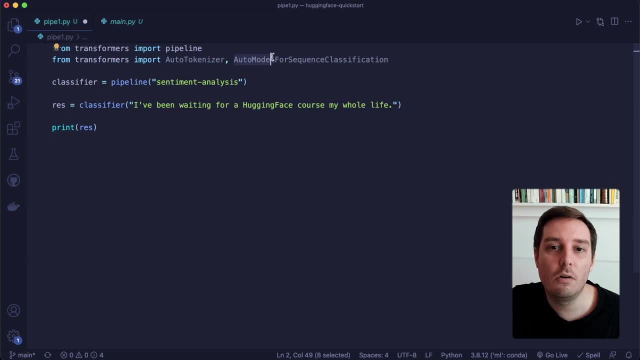 This one here is a very generic class, And this is also a generic class but a little bit more specified for the sequence classification task. So for this I just recommend to have a look at the official documentation. But for example, if you know you want a specific one, there's for. 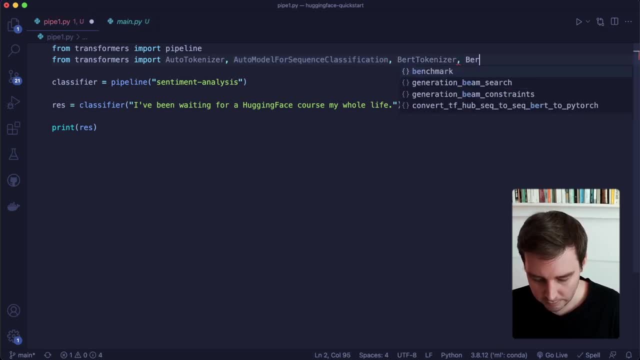 example, also a bird tokenizer class and a bird model class. So yeah, so we import those classes and then we create instances of this. So for this we specify a model name. So in this case this is just the default model that is used for this. 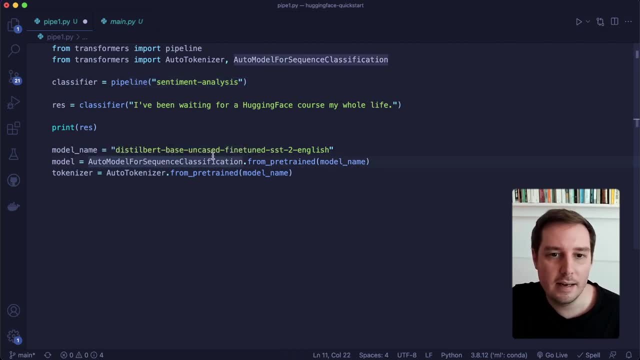 pipeline. And then we call the model class and say dot from pre trained, with the model name and the same for the tokenizer. And this from pre trained method is a very important method in hugging phase that you will see a lot of times, So just keep this one in mind. And now that we 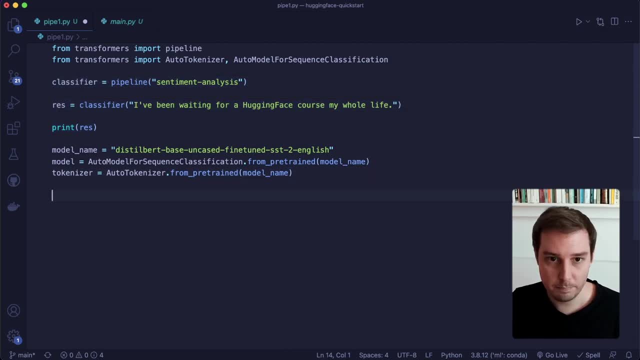 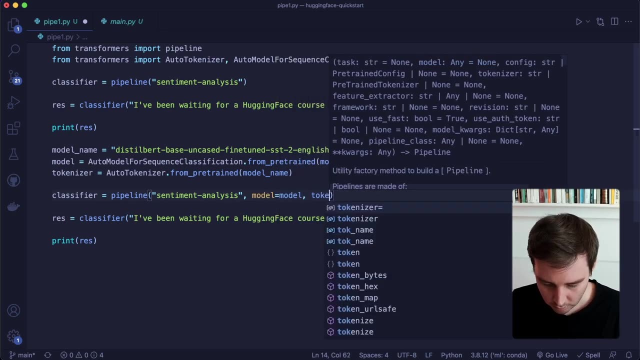 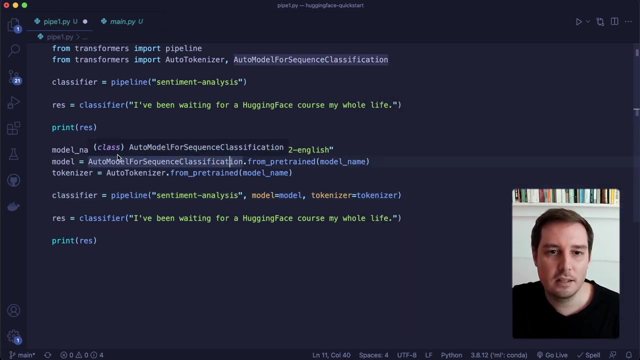 have this: we can, for example, copy and paste the same code. So let's say we want to copy and paste code And now for the pipeline, we can say: model equals model and tokenizer equals the tokenizer. And now, since this is just the same default model, this should produce the very same results. So 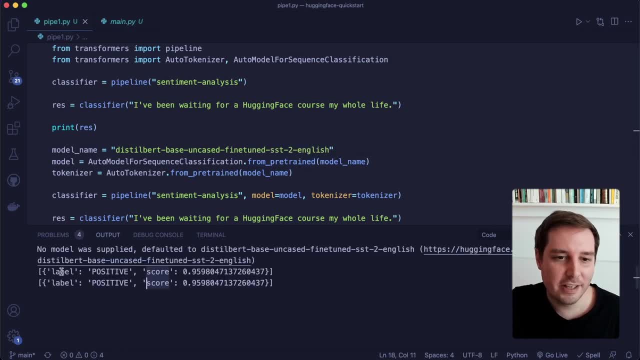 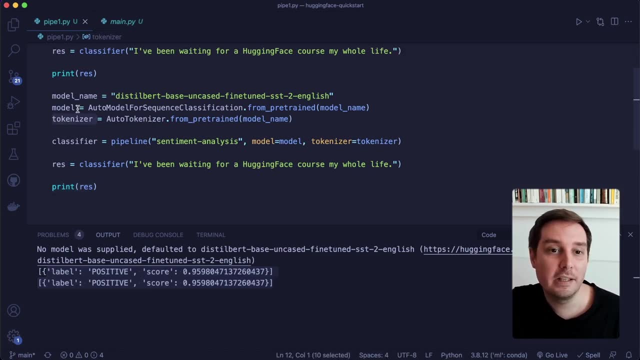 let's run this and have a look at the output, And the result is the very same, like I said, so this works. So, yeah, this is what's going on under the hood. So there will be a tokenizer and a tokenizer, And now let's have a look at the tokenizer and see what this is doing. So a 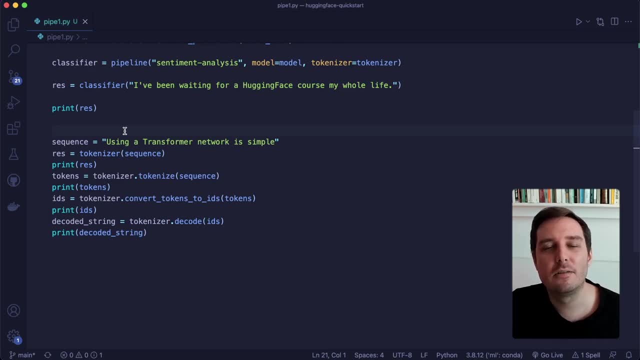 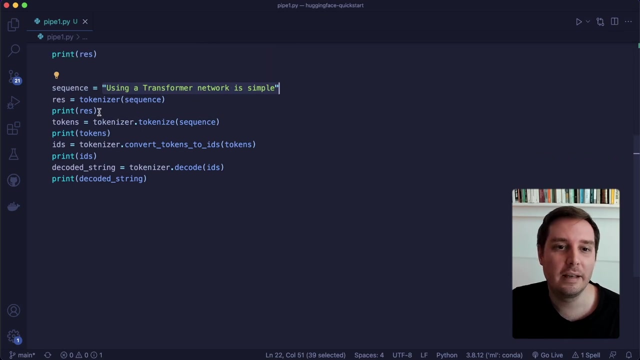 tokenizer basically puts a text in a mathematical representation that the model understands And in order to use this, we can call the tokenizer directly and give it a text as input, Or we can also put in multiple texts as once, as a list, And we can. so here we do this and print this. 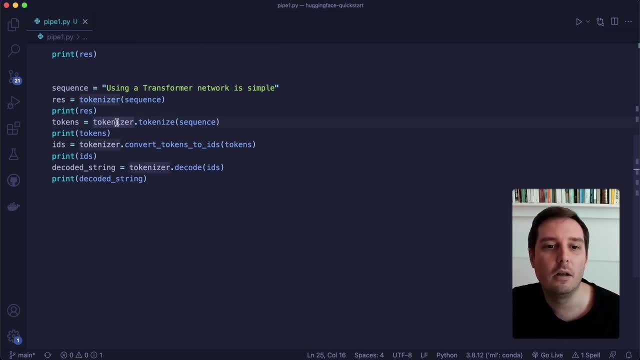 And we can also do this separately. So we can call tokenizer dot- tokenizer- tokenize. this will give us tokens. back then we can call tokenizer dots- converge tokens to IDs. this will give us the IDs, And we can do it the other way around, So we can 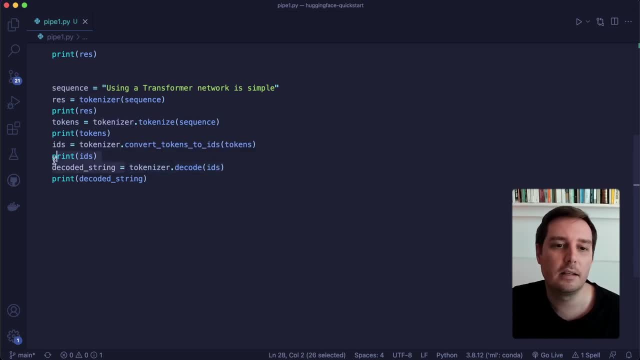 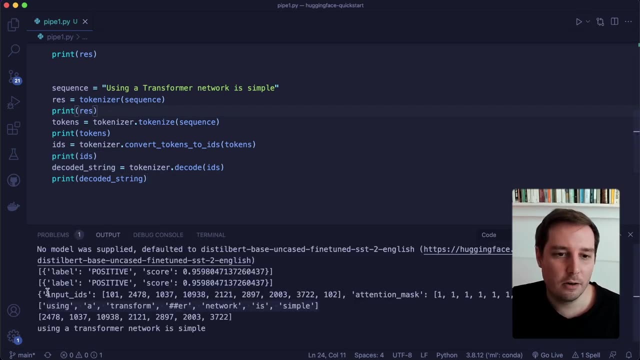 call tokenizer, dots, decode IDs, And this will give us the original string back. So let's run this and have a look at the different outputs. Alright, so here we see the output. So if we apply the tokenizer directly, then here we get this dictionary And the dictionary. 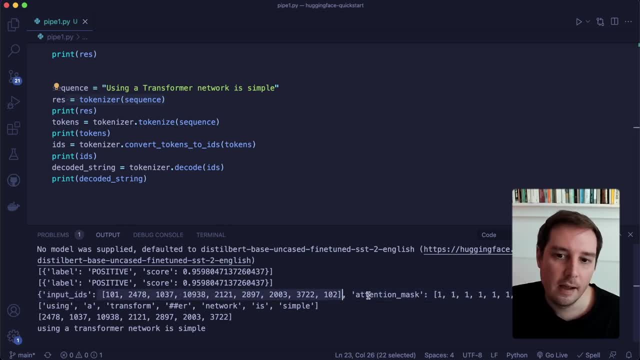 contains the input IDs that look like this, then we also have a attention mask, So for now we don't have to worry about this. A attention mask basically is a list of zeros and ones, and a zero means that the attention layer should ignore this token. Then if we 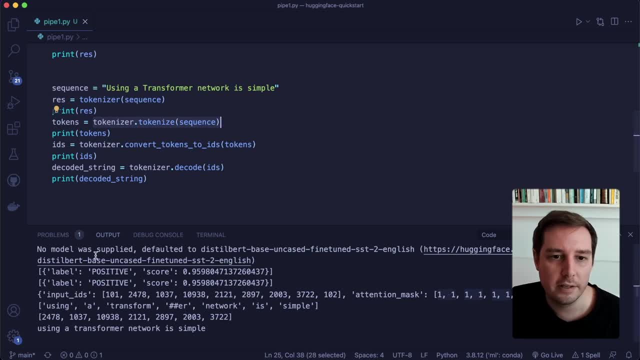 do this separately. so if we call tokenizer, dots, tokenize, then here we see the different tokens. then if we convert the tokens to IDs, then each token has a unique corresponding ID. So we see this here, And if we decode this, then we get the original string back. 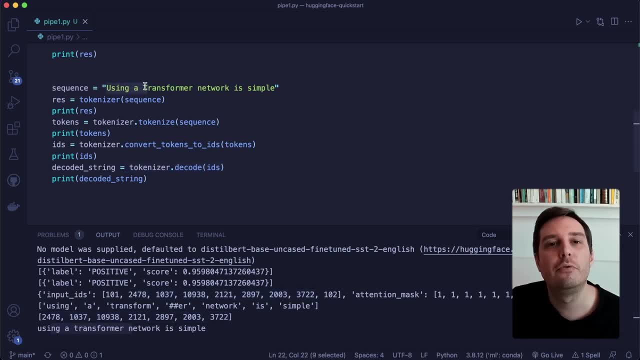 But here please note that we basically remove the capitalization. But yeah, and now if we compare this one with this one, then you see this should be the very same IDs, But here we also have this ID and this ID, So this means beginning of string And this one should. 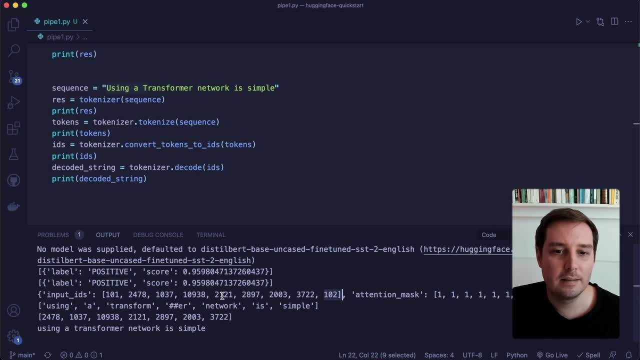 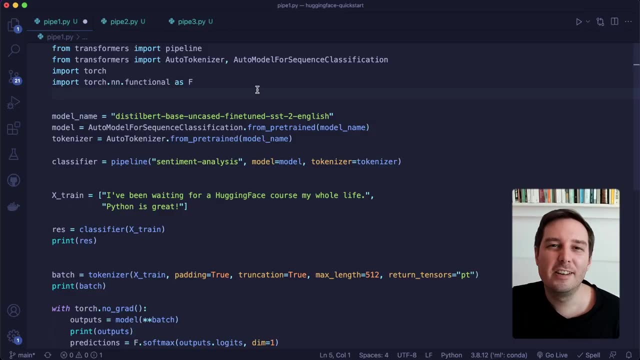 be the beginning of string, And this one should be the beginning of string, And this one should be the beginning of sentence and end of sentence. But basically, yeah, it's the same And yeah, and this is how a tokenizer works. Now let's see how we can combine the code with pytorch. 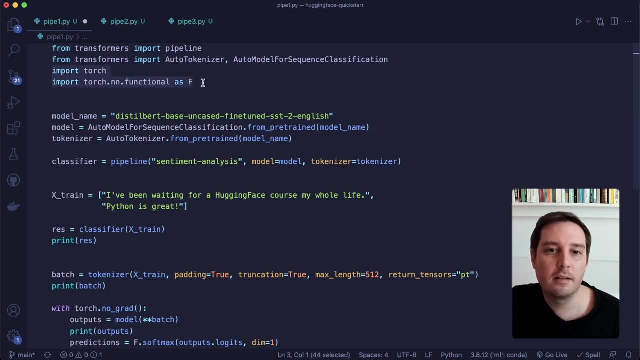 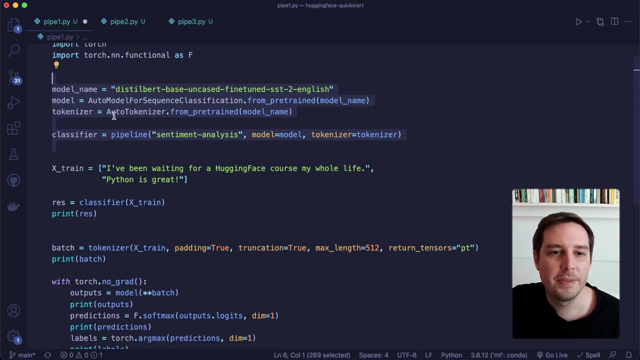 or TensorFlow. So in this example we use pytorch, But the code is very similar with TensorFlow. So with TensorFlow usually we have a TF before all those classes And yeah, in the first case I simply apply the pipeline like before. 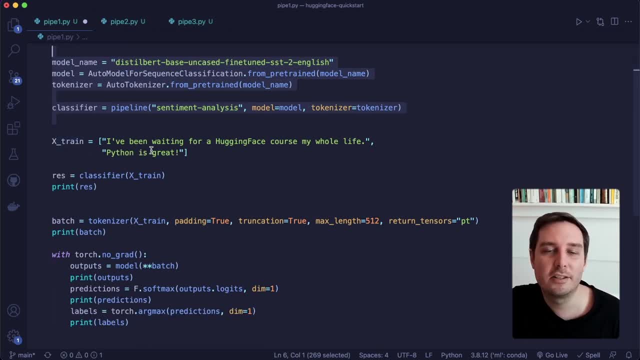 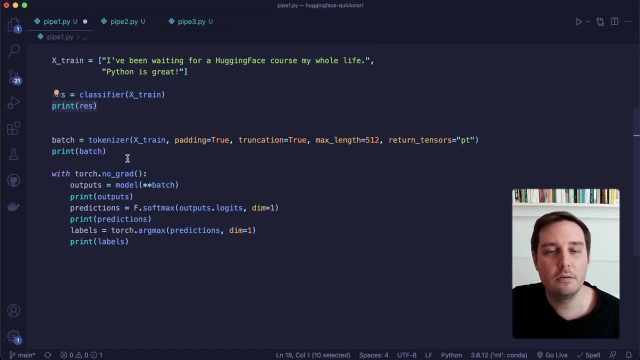 And now we use multiple sentences. So usually we just put in one sentence, But we can use a list of all those sentences. So we call this our x train data. And yeah, here we feed it to the pipeline classifier and print the result. And now we do this separately. So 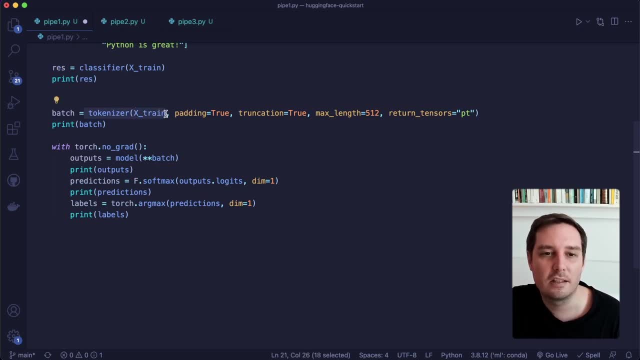 first we call the tokenizer with the X train data And we call this our batch, And then we can give it different arguments, like padding equals. And then we can call it a class, and like: padding equals true, truncation equals true. max length equals 512.. And return tensors. 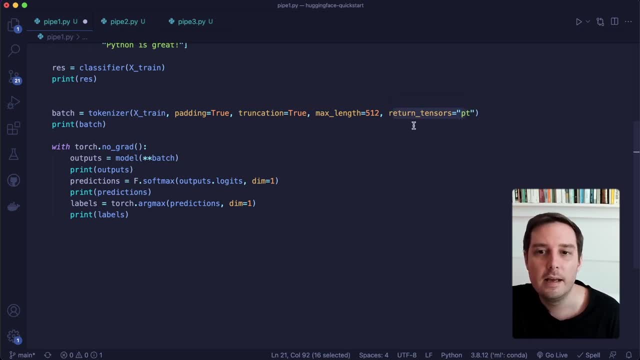 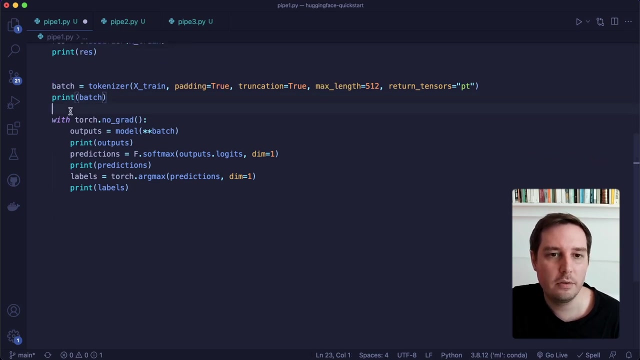 equals PT. So this will be in pytorch format. So you will see how this looks in a moment, because we print the batch. So, yeah, usually we apply the tokenizer directly, instead of doing the different functions separately, And then we do the inference in pytorch. So 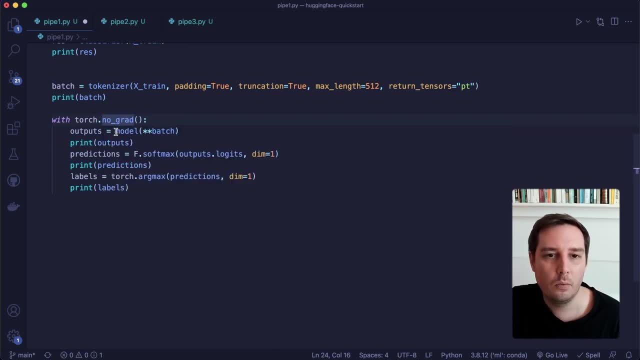 for this. we say: with torch dot no grad, then we call our model and here we unpack this batch, because this is a dictionary, And then we can apply different functions like f dot softmax to get the predictions, or torch dot arcmax to get the labels. And again these 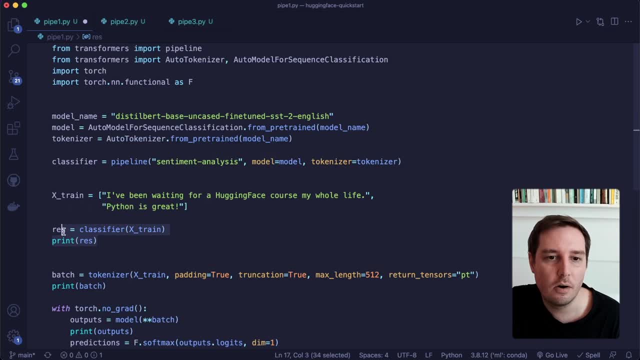 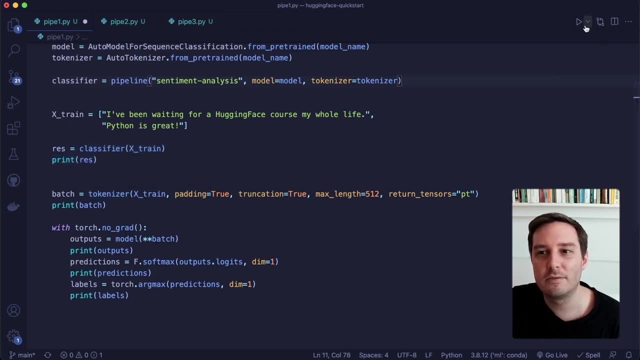 predictions should be the same scores that we get from our pipeline, because it essentially is the same step, except that now we do it for ourselves. So let's run this And have a look at the result. So yeah, here we print the batch and you see, this is a dictionary. 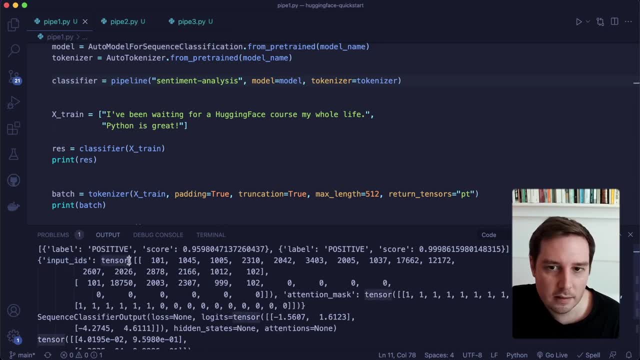 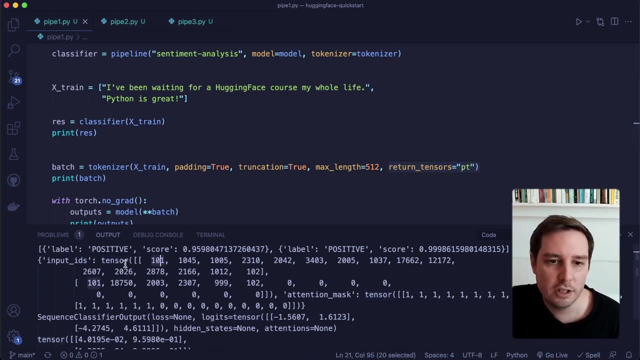 with the input IDs. And now we see this is a tensor And this is because we specified in pytorch tensor format. So without this this would just be a normal list, And then we had to take care of putting it in the correct format ourselves. But yeah, this makes it. 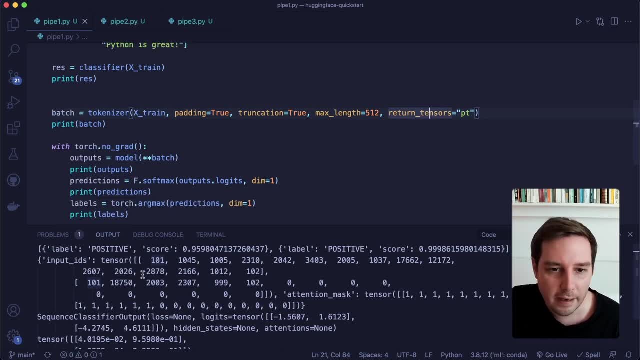 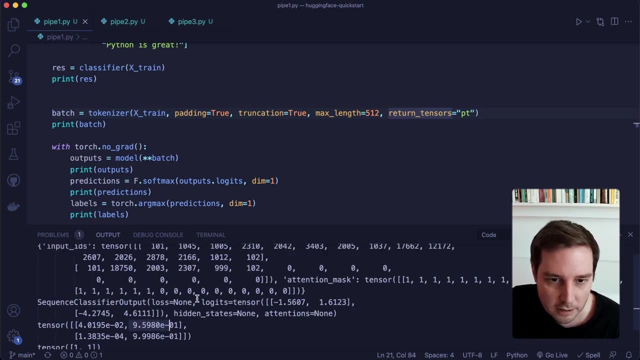 super handy to work with pytorch and TensorFlow, And then here we print the predictions, So let's do this, let's do this, And so we can see the results. So this is the batch and the labels. And you see, if we compare this prediction score with this one, then 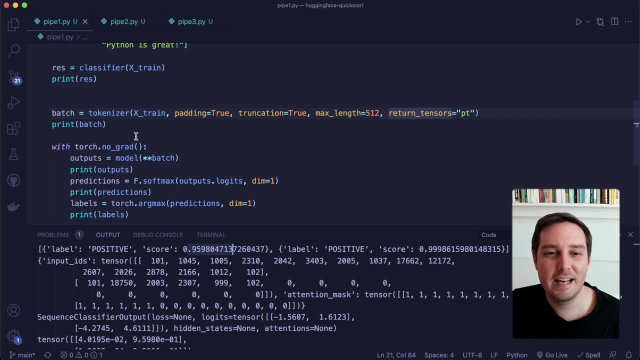 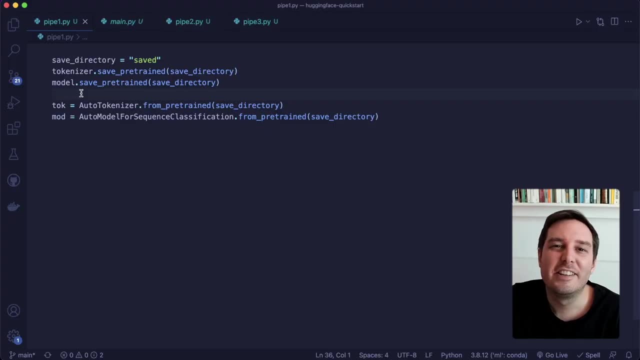 it's the very same. So, yeah, this is how it works. if we do it step by step, And this could be useful if we, for example, want to fine tune our model with a pytorch training loop, Not to save a tokenizer and model, we can specify a safe directory And then we can call tokenizer. 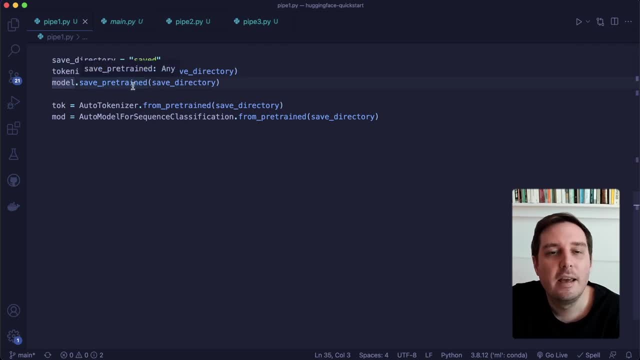 dot save pre trained and also model dot save pre trained. And when we want to load this we can pick a class like this one and then call auto tokenizer dot from pre-trained and Also for the model we say dot from pre-trained and then we get the loaded tokenizer and model and this should get you the same. 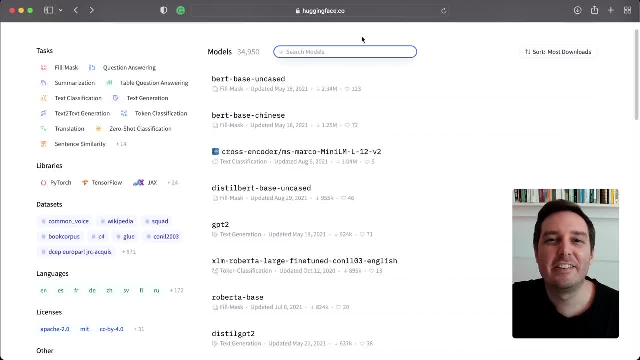 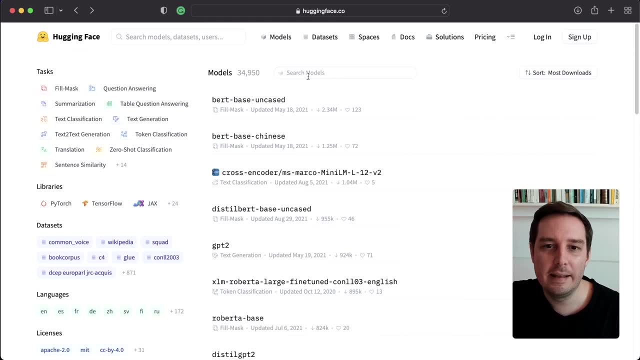 results as before. Now let's have a look at how we can use different models from the model hub. So on the official homepage we can click on models and then you see there are almost 35,000 models available created from the community, which is just awesome. 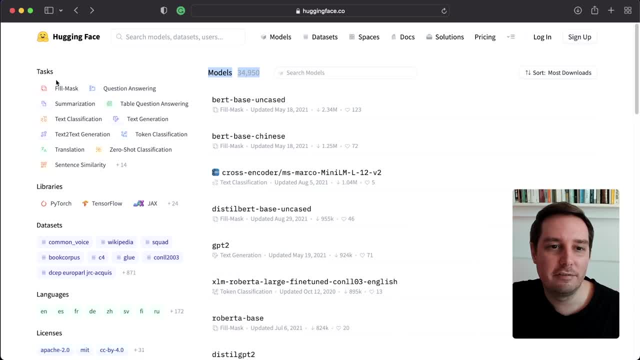 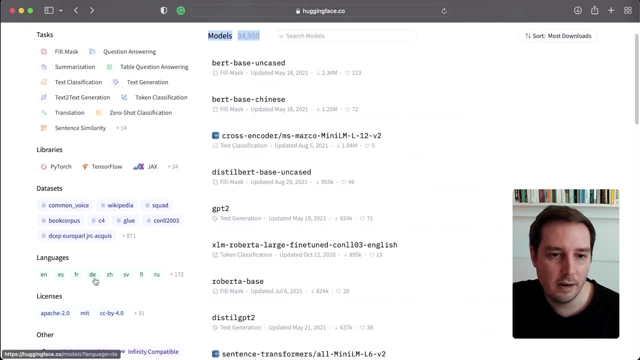 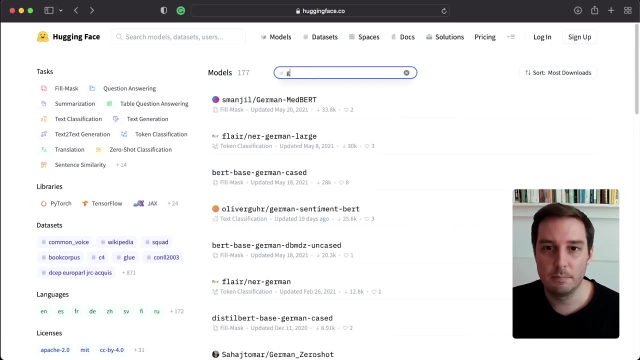 So here on the left side we can filter. for example, we can filter for the different pipeline tasks, or we can filter for libraries or data sets or languages, and We can also use the search bar. For example, if I want a German model, I can simply search for this. 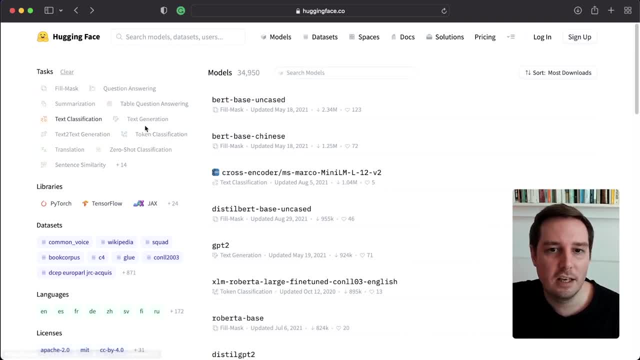 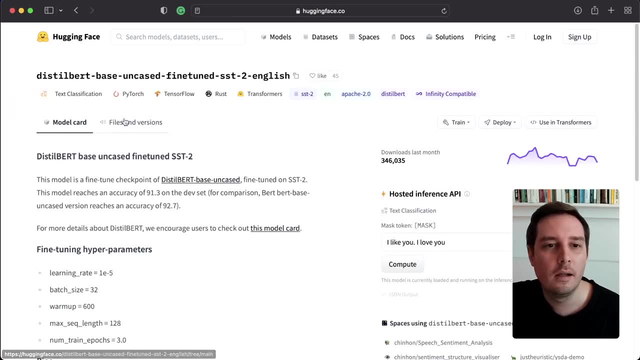 So here let's filter for text classification. So this is the same as the text analysis task and in this case this is the default model and Usually the name says the name of the models. in this case It's a distal bird based uncased model, and then it's fine-tuned on the sst2 data set and it's in English. 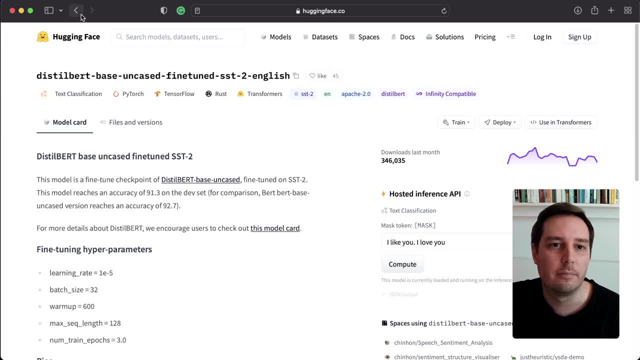 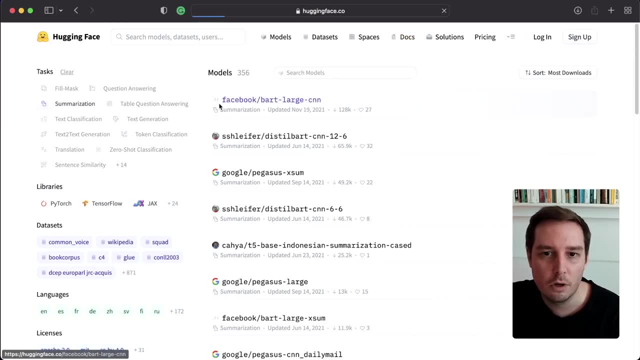 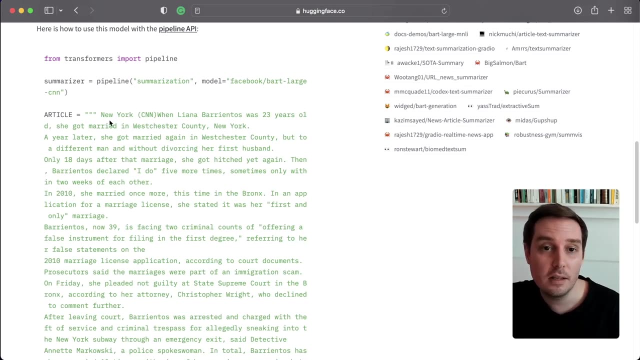 So yeah, and then you can read through this and find out more information. so let's, for example, clear this and search for summarization and then click on this one and Yeah, sometimes you even find code examples. and the way you can use this now is either you grab the code example or